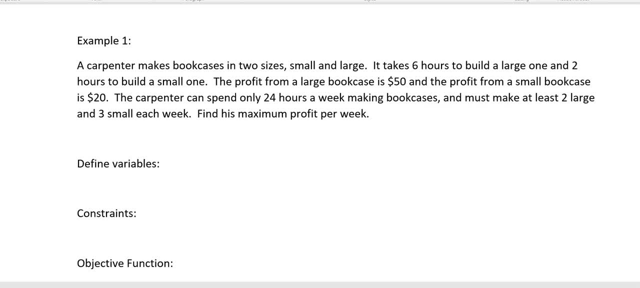 talk about. first of all, what is it? Linear programming is a name for a you know, something we do in math. that really means almost nothing. It makes no sense, you know. it doesn't tell you what it is, So let's talk about what it actually is. It's basically word problems that you are. 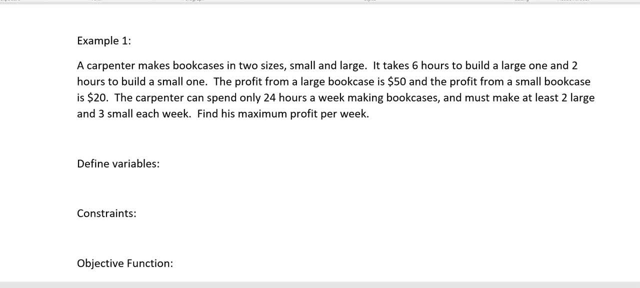 trying to solve and what you're usually trying to find is you're trying to find a minimum, or a maximum like maybe the maximum profit you could make or the minimum amount of packaging that you could have to use to package something that you're going to ship, or something like that. So you're 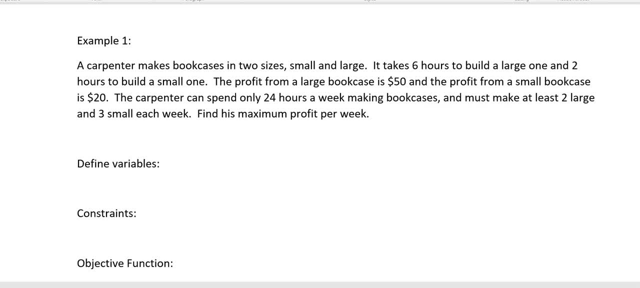 trying to figure out what values of the variables will help you to maximize or minimize something, and that means another word for doing both of those in other words we sometimes use is to optimize, In other words, to make the most of it, or the best situation, The best situation. 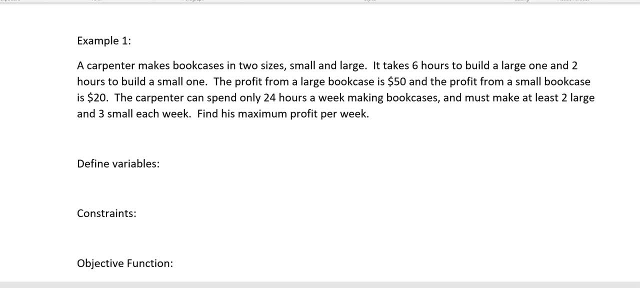 could be the maximum profit or the minimum amount of packaging. So generally it's pretty much just word problems where you're trying to optimize something, and these are actually pretty common in business. So the first example here that I'm showing you says a carpenter makes bookcases in. 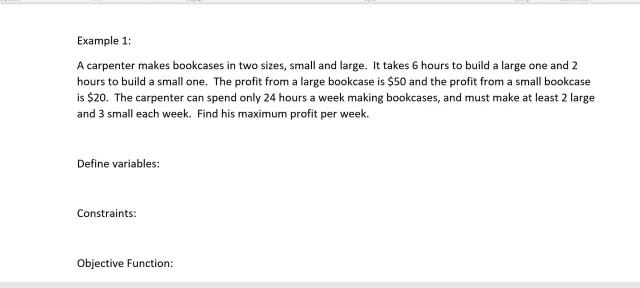 two sizes: small and big. Small and large. It takes six hours to build a large one and two hours to build a small one. The profit from a large bookcase is $50, and the profit from a small bookcase is $20. 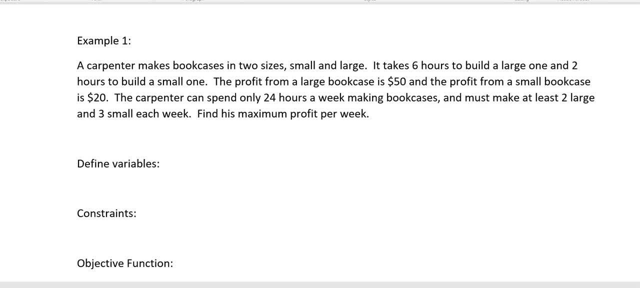 The carpenter can spend only 24 hours a week making bookcases and must make at least two large and three small each week. Find his maximum profit per week. So there's a lot of information in there and that's very common for a linear programming problem. There's a lot of information in 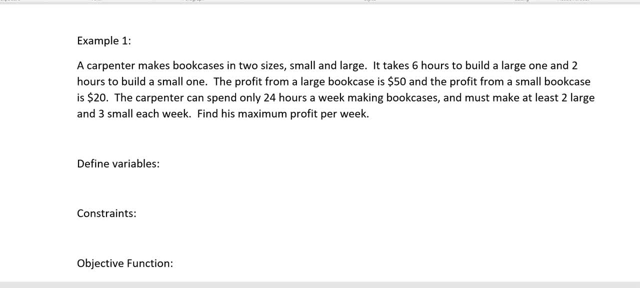 sort of a short paragraph and if you try to just go through it and like as you were reading it, write equations or something, that would be very difficult, or at least it would be for me, To me the easiest way to do this- and these things right down here define your variables. 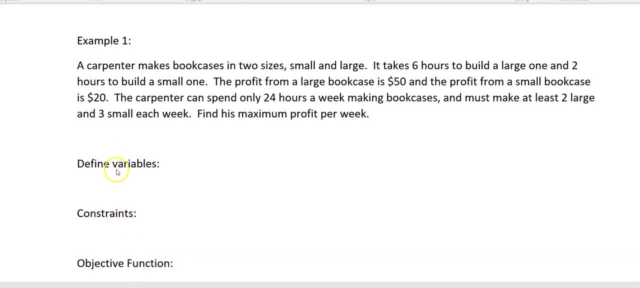 and constraints in an objective function. these are what you're going to be asked for on your first homework assignment on. this is the first homework assignment you're doing really doesn't take it all the way to the end of the problem, It's just finding these things. So to me, when it 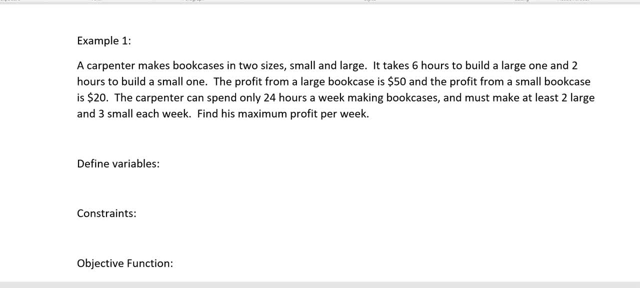 sort of a short paragraph and if you try to just go through it and like as you were reading it, write equations or something, that would be very difficult, or at least it would be for me, To me the easiest way to do this- and these things right down here define your variables. 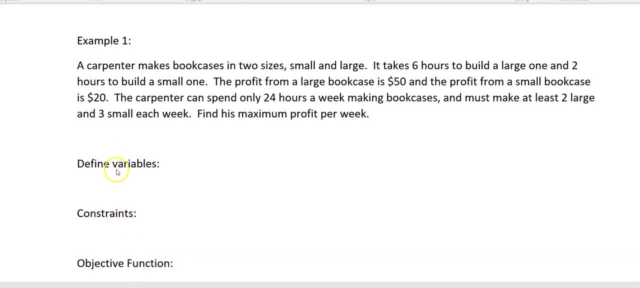 and constraints in an objective function. these are what you're going to be asked for on your first homework assignment on. this is the first homework assignment you're doing really doesn't take it all the way to the end of the problem, It's just finding these things. So to me, when it 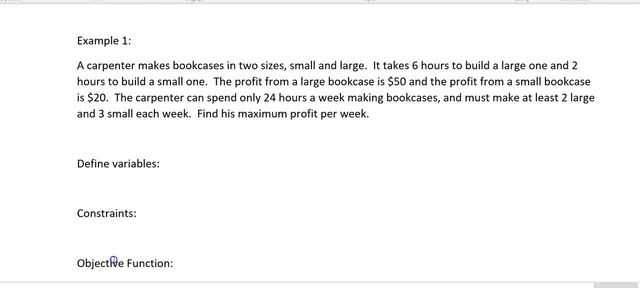 comes to finding these things, the easiest thing to find is this. first, If it'll let me, there we go. The objective function is basically the function. It's- excuse me, It's like an expression for the thing that you are trying to maximize or minimize. Sometimes people call it the profit function. If 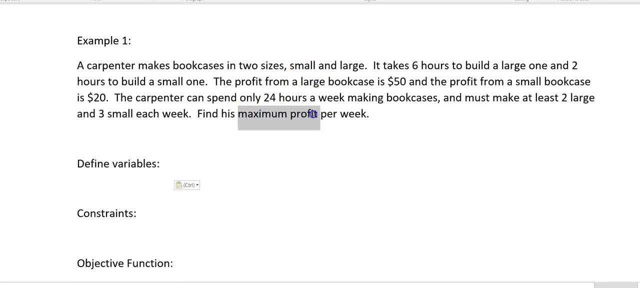 we're trying to get a maximum profit, like we are here, which is pretty common, Okay, But the objective function is: it's kind of: what is your objective? Your objective is to maximize something or to minimize something, So you need an expression for whatever. 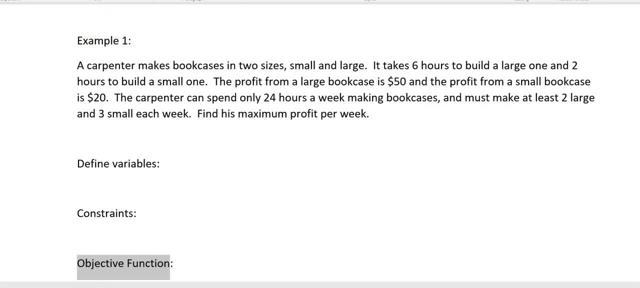 it is you're trying to maximize or minimize. Very often the information about whatever you want to try to maximize or minimize is found at the end of the problem or at the end of the paragraph. So, basically, the last thing they do generally is tell you what you're going to. 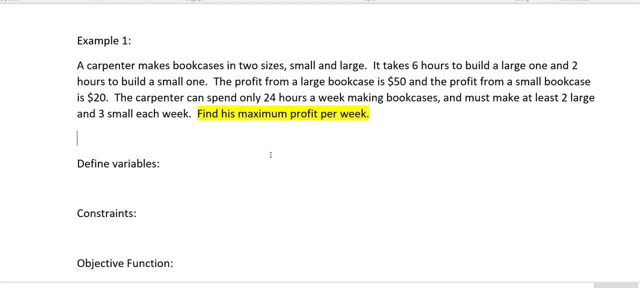 minimize. So here they told me I need to maximize the carpenter's profit. Okay, So it says per week, but everything here is based on only a week, pretty much how much time there is in a week, and that kind of thing. So find his maximum profit. So that's what I have to do, is I have to find the maximum. 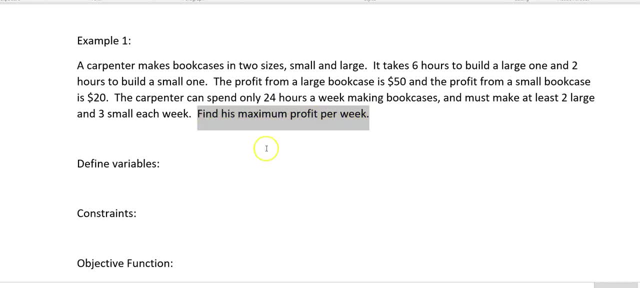 profit, And so that means a, an expression for his profit is going to be what the objective function is. So it's kind of like: okay, how would you find his profit? Well, what would I have to know? Um, look, first of all, profit is money. 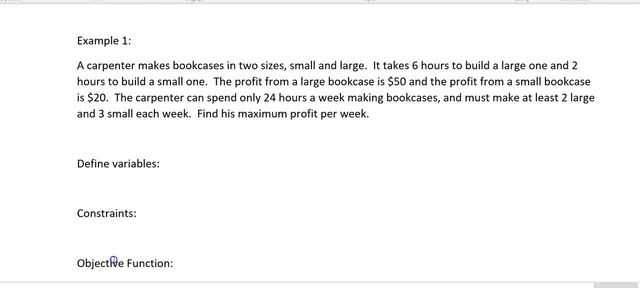 comes to finding these things, the easiest thing to find is this. first, If it'll let me, there we go. The objective function is basically the function. It's- excuse me, It's like an expression for the thing that you are trying to maximize or minimize. Sometimes people call it the profit function. If 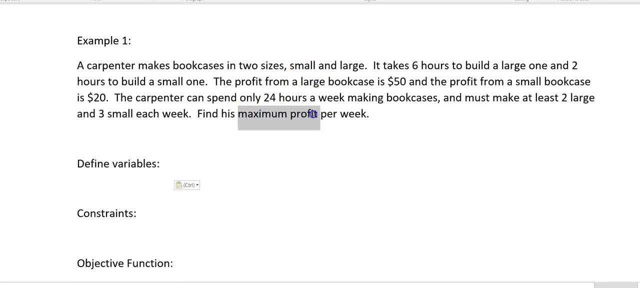 we're trying to get a maximum profit, like we are here, which is pretty common, Okay, But the objective function is: it's kind of: what is your objective? Your objective is to maximize something or to minimize something, So you need an expression for whatever. 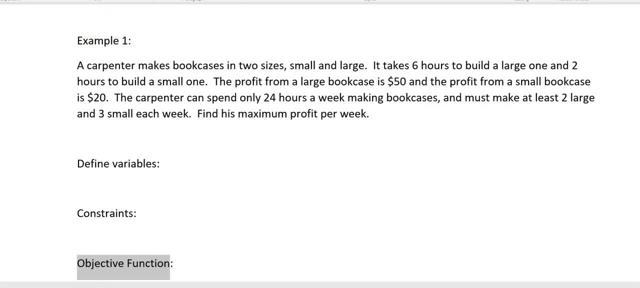 it is you're trying to maximize or minimize. Very often the information about whatever you want to try to maximize or minimize is found at the end of the problem or at the end of the paragraph. So, basically, the last thing they do generally is tell you what you're going to. 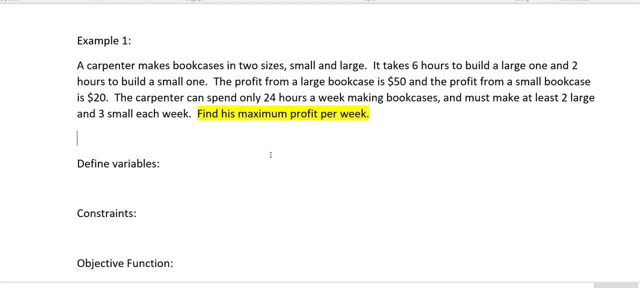 minimize. So here they told me I need to maximize the carpenter's profit. Okay, So it says per week, but everything here is based on only a week, pretty much how much time there is in a week, and that kind of thing. So find his maximum profit. So that's what I have to do, is I have to find the maximum. 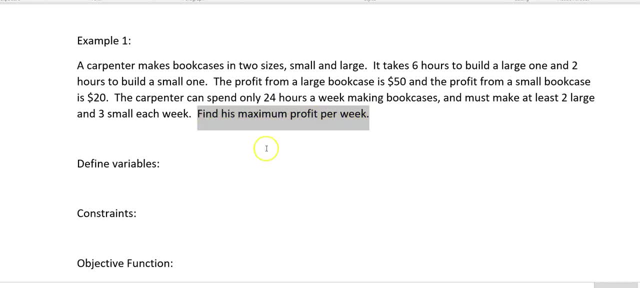 profit, And so that means a, an expression for his profit is going to be what the objective function is. So it's kind of like: okay, how would you find his profit? Well, what would I have to know? Um, look, first of all, profit is money. 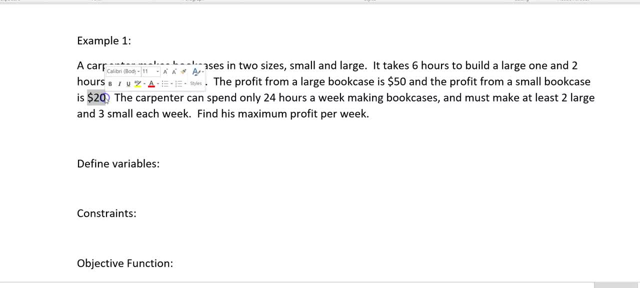 So here's something about money and here's something about money. So this is guiding me into what do I look back into the problem and find? So I've got two things about money. I know that a large bookcase is $50.. I know that a small bookcase is $20. and that's profit. That's not just. 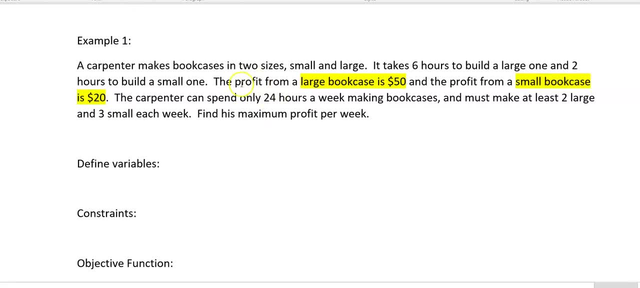 like the total price. That's the profit. So those two are about the profit. So if I can figure out how to write an expression that would describe his profit, that's going to be my objective function. If I knew how many large bookcases he made and how many small bookcases he made, I would know it. 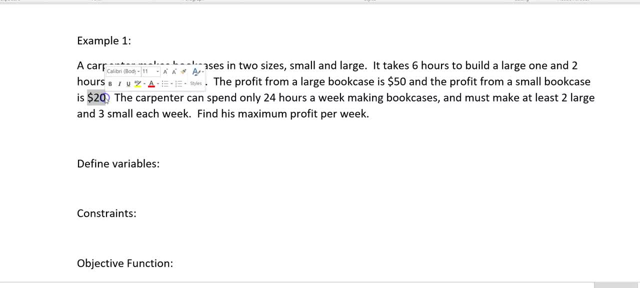 So here's something about money and here's something about money. So this is guiding me into what do I look back into the problem and find? So I've got two things about money. I know that a large bookcase is $50.. I know that a small bookcase is $20. and that's profit. That's not just. 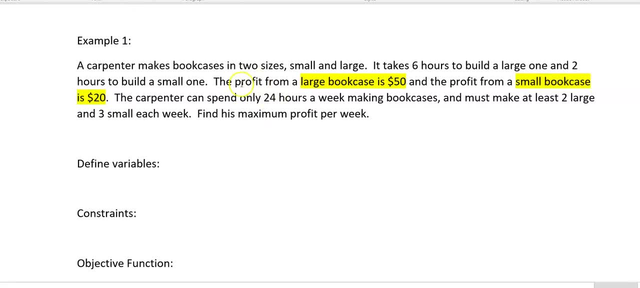 like the total price. That's the profit. So those two are about the profit. So if I can figure out how to write an expression that would describe his profit, that's going to be my objective function. If I knew how many large bookcases he made and how many small bookcases he made, I would know it. 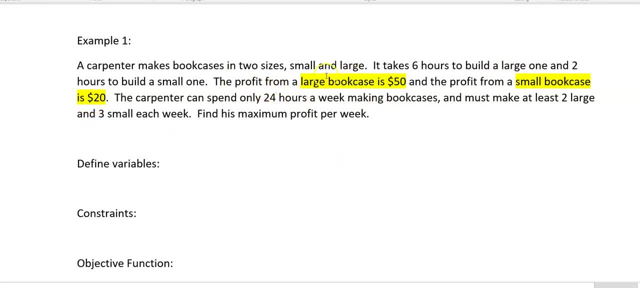 Like if he made three large bookcases and three small bookcases, I would say three times 50 and three times 20.. So, basically, what this does is not only tell me what is my objective function, but it has given me a big clue as to what my variables are going to be. 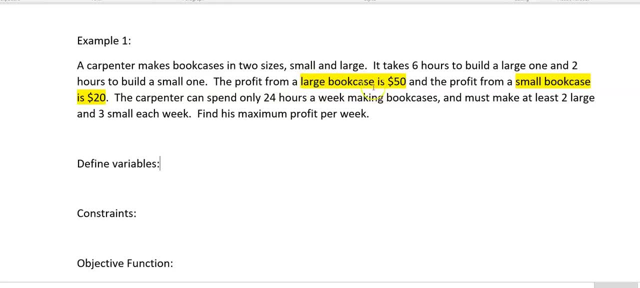 In other words, I need to find out how many large bookcases he's making and I need to find out how many small bookcases he's making, And that would give me the profit. So I'm going to let L stand for large, and it's not just going to stand for large in general, It's. 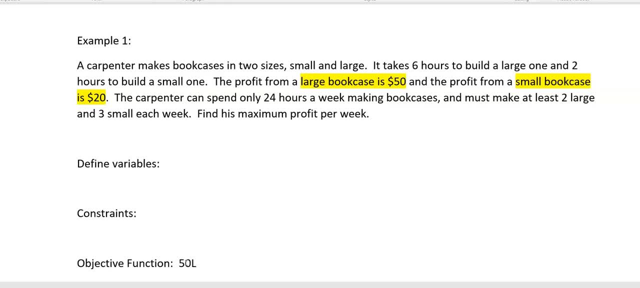 going to stand for the number of large bookcases he's making And I'm going to let S stand for the number of small bookcases he's making. You can use X and Y, And when we get to the graph I may decide that I wish I had, But for right now we're going to go ahead and use L, for large is for the. 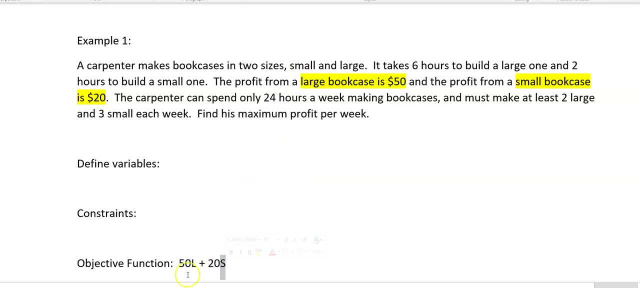 number of large bookcases. S is for the number of small bookcases, And if I could know those and plug them in, then that would give me my objective function. So notice, this is just an expression. There's no equal sign, because I don't know what that's going to equal. It's just something that 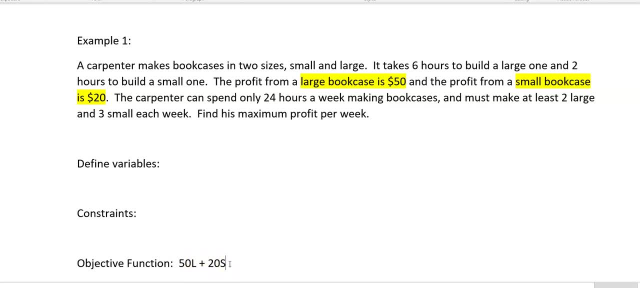 I would plug into to find out what is my maximum profit once I have some values there for how many large bookcases and how many small bookcases he's going to make So variables. we said L is the number of large bookcases he's making Built, I guess, And S is the number of small bookcases built. 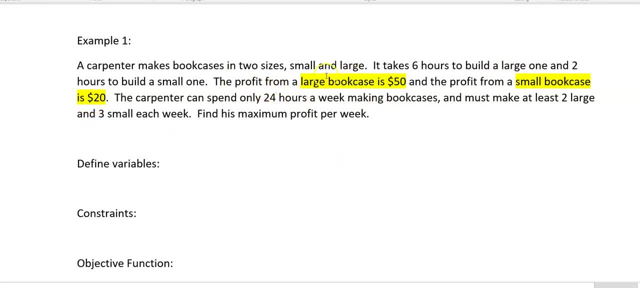 Like if he made three large bookcases and three small bookcases, I would say three times 50 and three times 20.. So, basically, what this does is not only tell me what is my objective function, but it has given me a big clue as to what my variables are going to be. 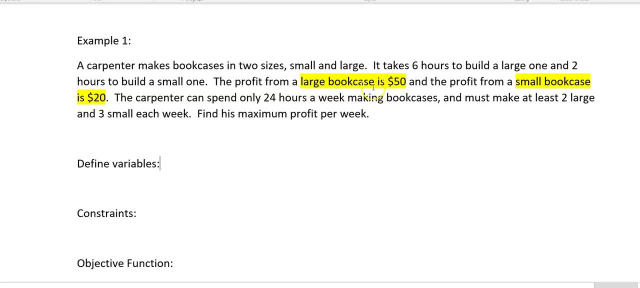 In other words, I need to find out how many large bookcases he's making and I need to find out how many small bookcases he's making, And that would give me the profit. So I'm going to let L stand for large- and it's not just going to stand for large in general. 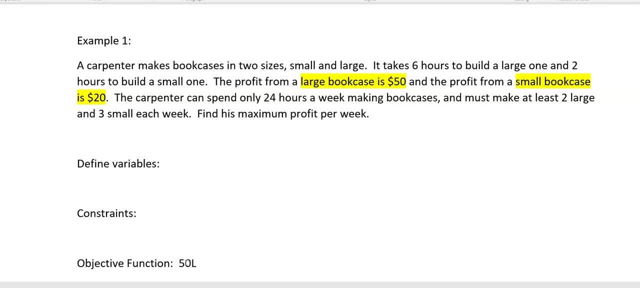 it's gonna stand for the number of large bookcases he's making And I'm going to let S stand for the number of small bookcases he's making. You can use X and Y, And when we get to the graph, I may. 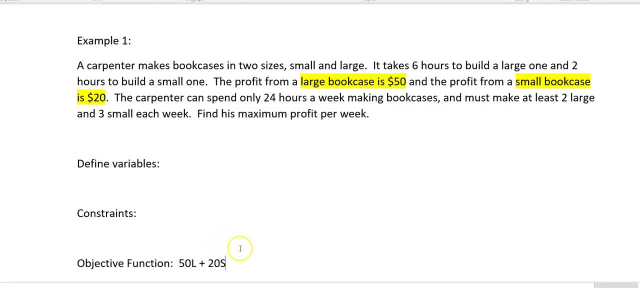 decide that I wish I had, But for right now we're going to go ahead and use: L for large is for the number of large bookcases, S is for the number of small bookcases, And if I could know those and plug them in, then that would give me my objective function. So notice, this is just an expression. 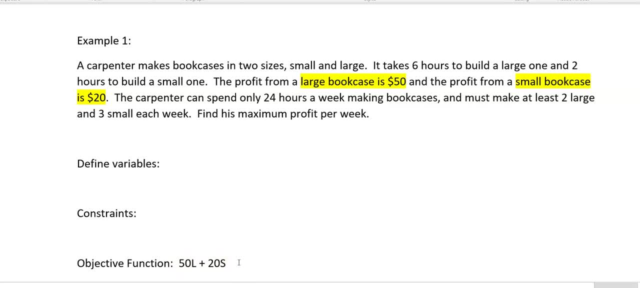 There's no equal sign because I don't know what that's going to equal. It's just something that I would plug into to find out what is my maximum profit Once I have some values there for how many large bookcases and how many small bookcases he's going to make, So variables. we said L is. 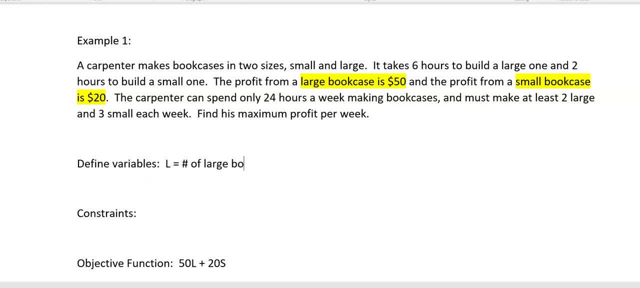 the number of large bookcases he's making Built, I guess, And S is the number of small bookcases built. Okay, so again, I started by looking at the very end. what are you asking me to optimize, to maximize or minimize? And then I went back and I figured out where that information was. 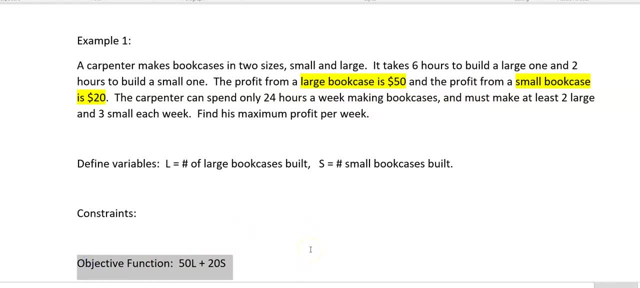 and wrote the objective function using that information, And in doing so, that helped me figure out what was it that I needed my variables to be about. Okay, the number of large bookcases built and the number of small bookcases built. Now the constraints. these are basically your limitations, And the rest of the problem is: 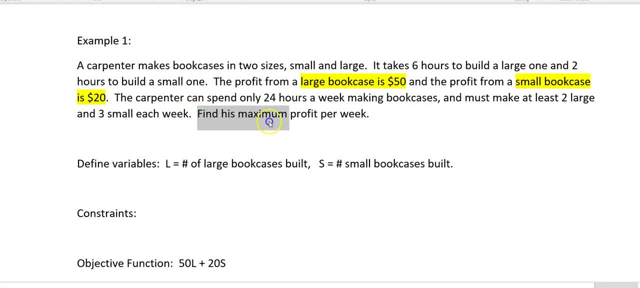 Okay, so again, I started by looking at the very end: What are you asking me to optimize, to maximize or minimize? And then I went back and I figured out where that information was and wrote the objective function using that information And in the end I got the objective function And I 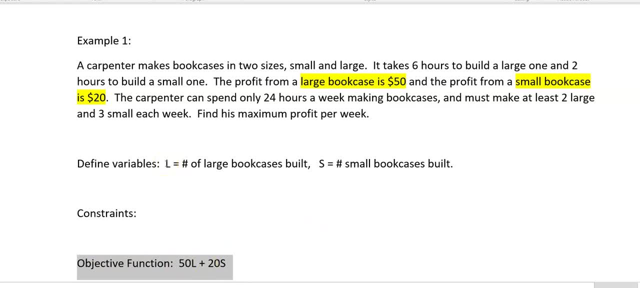 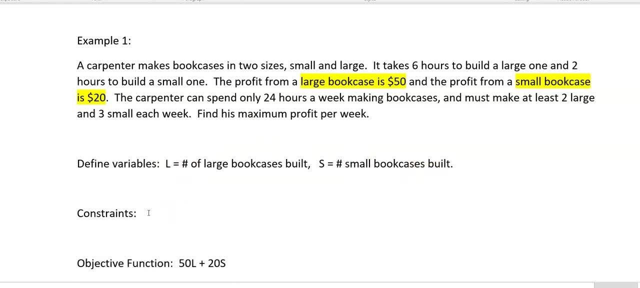 built. Now the constraints, these are basically your limitations, And it's the rest of the problem is giving you these, And they're all going to be inequalities, Things like: at least tell me that it's going to be greater than or equal to something. At most would be greater than or less. 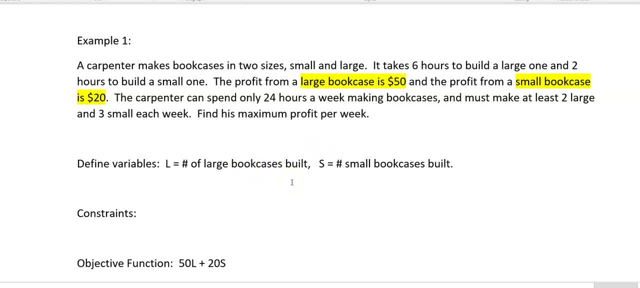 than. So I mean, excuse me, it would be less than or equal to. So those are the kinds of situations I'm doing. All of your constraints are always going to be inequalities. So he can only spend 24 hours per week. He must make at least two and at least. 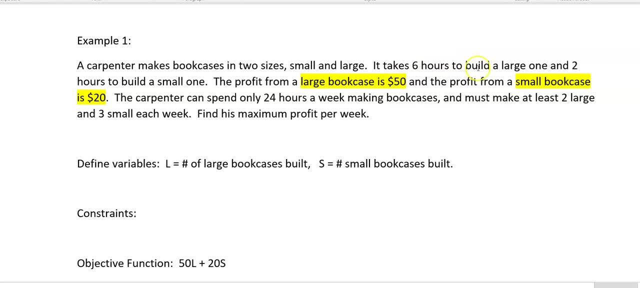 small, three small each week. It takes six hours to make a large one and two hours to make a small one. Okay, So if it takes him six hours for each large one, because large is the number of, I mean, L is the number of large bookcases, plus two hours for each. 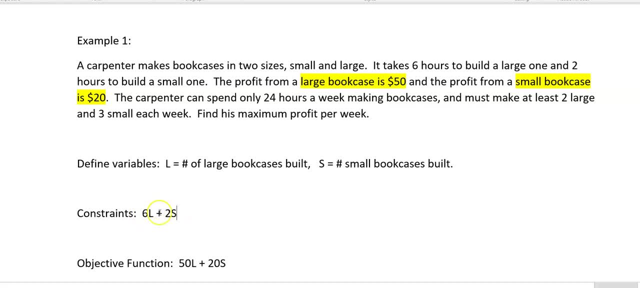 small one. Then basically, this describes how much time he's using: Six hours per the number of large bookcases, plus two hours per the number of small bookcases, And we know that he only has 24 hours. So there's a constraint. I'll say is less than or equal to, and I'm going to be lazy and just say: 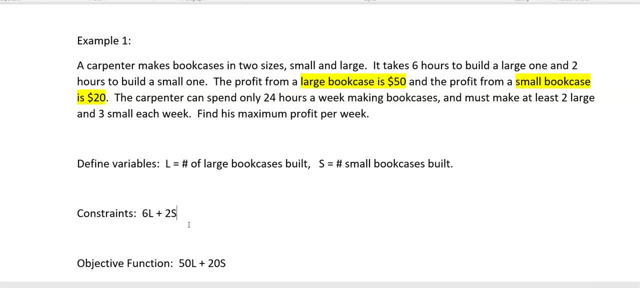 less than or equal to. if I were doing this, Oh, maybe I can do it. Let's see. Is less than or equal to 24.. So let's see if I can find the symbol. I was going to be lazy, but it's not working out too well. There we go. Okay, Is less. 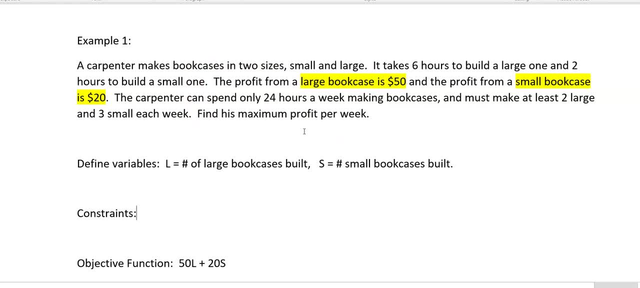 giving you these, And they're all going to be inequalities. Things like: at least tell me that it's going to be greater than or equal to something. At most would be greater than or less than some. I mean, excuse me, it would be less than or equal to. 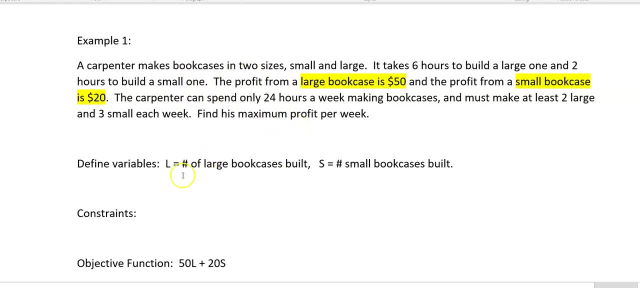 Um, so those are the kinds of situations I'm doing of. all of your constraints are always going to be inequalities. So he can only spend 24 hours per week. He must make at least two and at least small, three small each week. 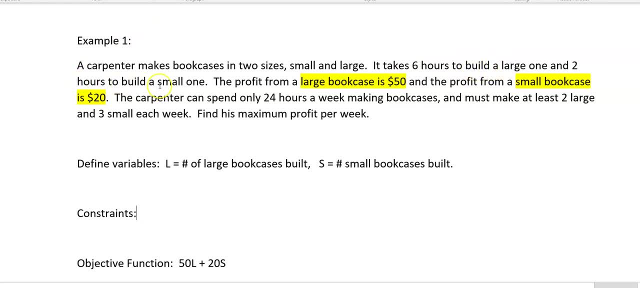 It takes six hours to make a large one and two hours to make a small one. Okay, so if it takes him six hours for each large one, cause: large is the number of bookscase built. the number of I mean L is the number of large bookcases, plus two hours for each small one. 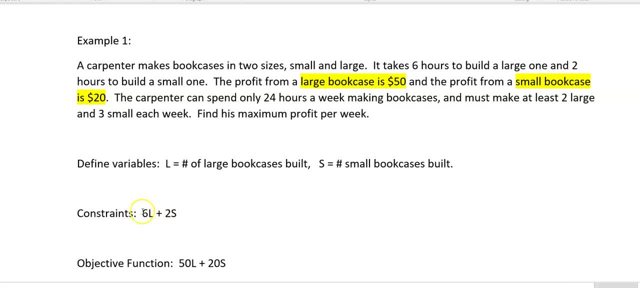 then, basically, this describes how much time he's using: Six hours per the number of large bookcases plus two hours per the number of small bookcases, And we know that he only has 24 hours. so there's a constraint. I'll say is less than or equal to, and I'm going to be lazy and just say less than. 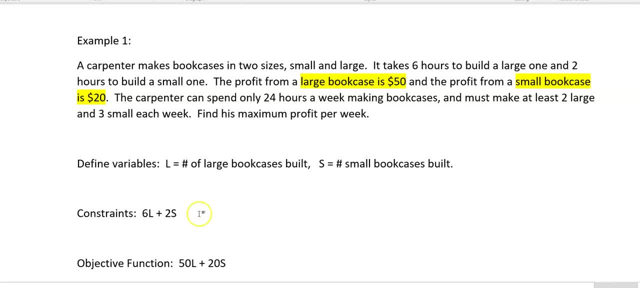 or equal to. if I were doing this, maybe I can do it. Let's see. Is less than or equal to 24.. Let's see if I can find the symbol. It's going to be lazy, but it's not working out too well. 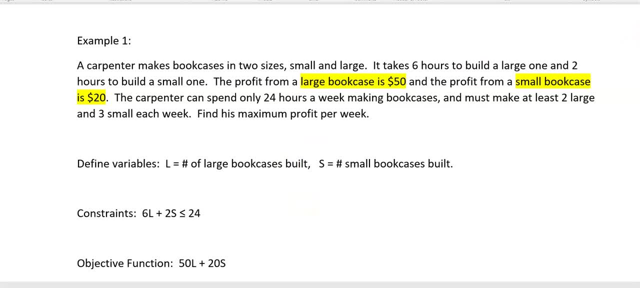 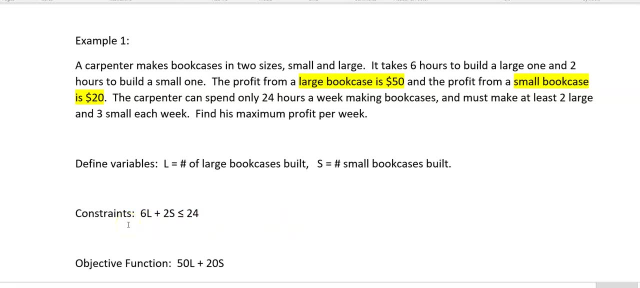 There we go. Okay Is less than or equal to 24.. All right, There's one constraint. You're usually going to have three or four constraints, Okay? Another constraint here, and I'm just going to give some space. Another constraint here is he has to make at least two large and three small each week. 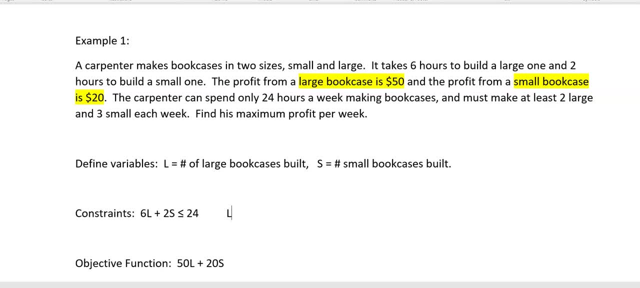 So the number of large has to be greater than or equal to two. So there's another inequality, That's another constraint, And the number of small has to be greater than or equal to two, Three, Okay, So let's go back through at this point and read everything and make sure we have 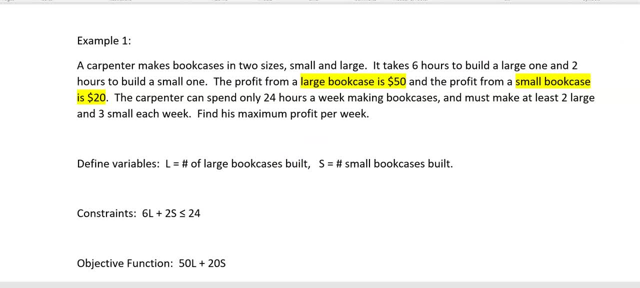 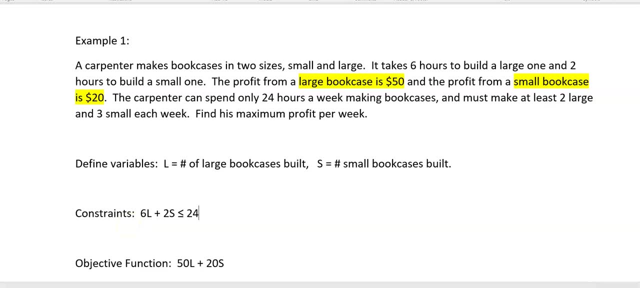 than or equal to 24.. All right, There's one constraint. You're usually going to have three or four constraints, Okay, Another constraint here, and I'm just going to give some space. Another constraint here is he has to Make at least two large and three small each week, So the number of large has to be. 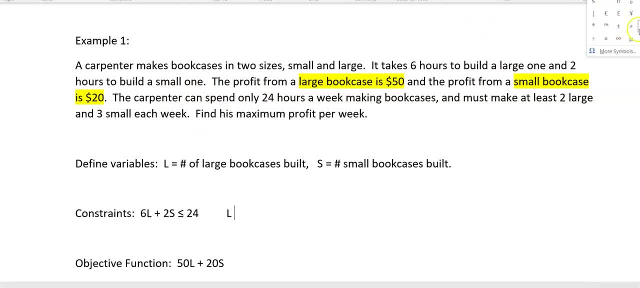 greater than or equal to two. So there's another inequality, That's another constraint, And the number of small has to be greater than or equal to three. Okay, So let's go back through at this point and read everything and make sure we have used all. 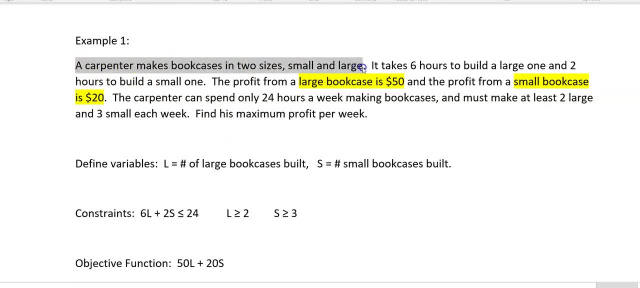 the info we have. This is just general info. Six hours to build a large and two hours to build a small. We've already talked about that and we know that that has to add up to less than 24 hours. Seriously, Seriously. 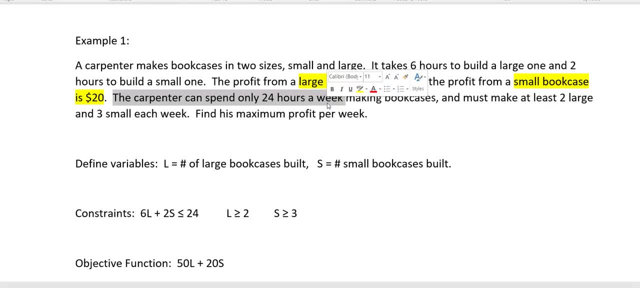 Seriously Come here. What's your problem? Okay, I don't know what the dog is barking at, but we'll find out. Okay, Yeah, I hear you. Um, let me see if I can pause. Okay, Sorry about that. The dog is now outside. 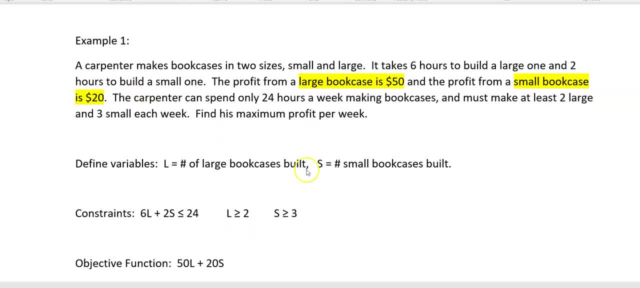 Okay, So basically, I just am checking back through to make sure I've covered everything and I have. So this is the stuff I need. I have to define my variables, I have to figure out what the constraints are and I have to figure out what the objective function is. Okay, This is all you're. 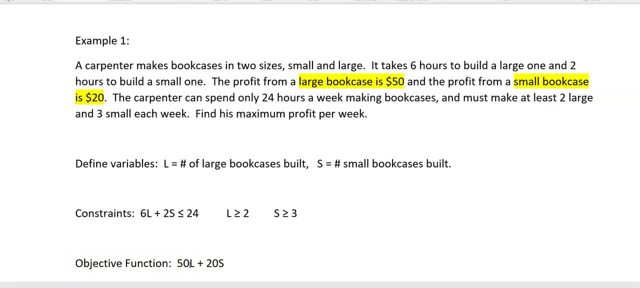 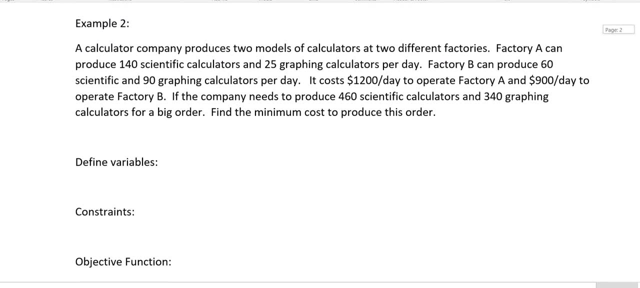 doing in your first night homework, All right. So let's go ahead and do that for one more example and then we'll pick up the next one. All right, So here, I will pick up here And do the rest of it tomorrow. 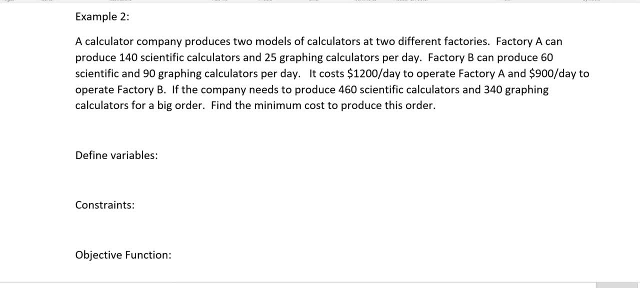 All right. example two: Let me give you some time to read that over. Actually, I guess I might as well related allowed to a calculator. Company produces two models of calculators at two different factories. Factory A can produce 140 scientific calculators and 25 graphing calculators per day. 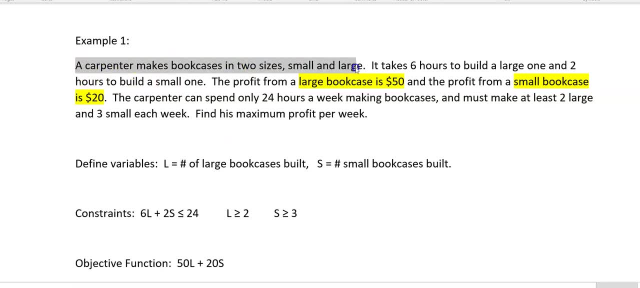 used all the info we have. This is just general info. Six hours to build a large and two hours to build a small. We've already talked about that and we know that that has to add up to less than 24 hours. Seriously, Seriously, Seriously. Come here. What's your problem? Okay, I don't know what. 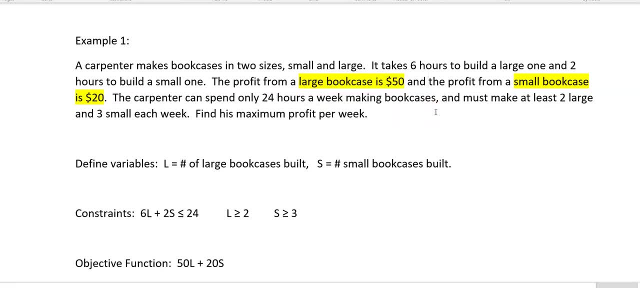 the dog is barking at, but we'll find out. Okay, Yeah, I hear you. Let me see if I can pause. Okay, Sorry about that. The dog is now outside, Okay. So basically, I just am checking back through to make sure I've covered everything. 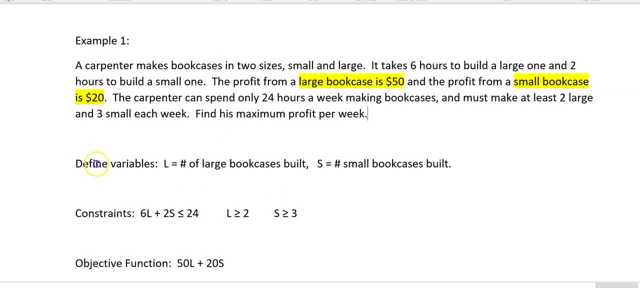 and I have. So this is the stuff I need. I have to define my variables, I have to figure out what the constraints are, and I have to figure out what the objective function is. Okay, This is all you're doing in your first night homework, All right? So let's go ahead. 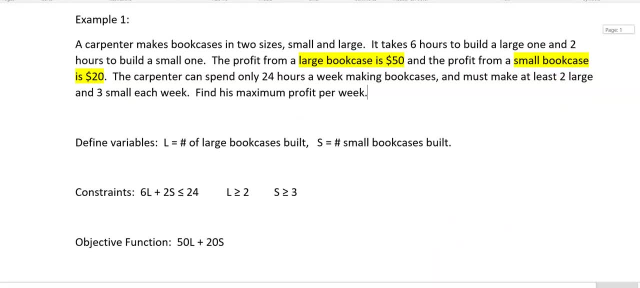 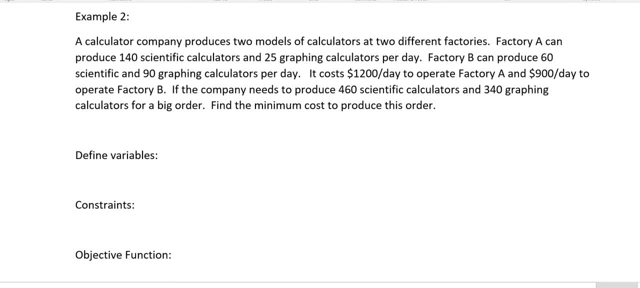 and do that for one more example, And then we'll pick up here and do the rest of it tomorrow. All right, Example two: Let me give you some time to read that over. Actually, I guess I might as well read it aloud too. A calculator. 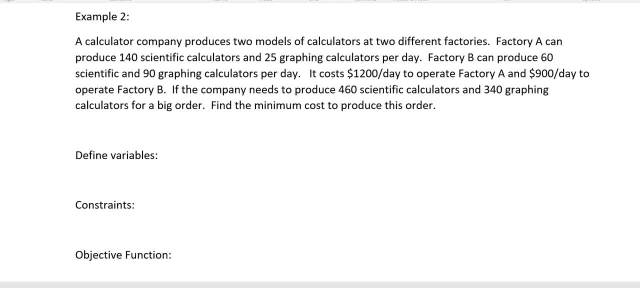 company produces two models of calculators at two different factories. Factory A can produce 140 scientific calculators and 25 graphing calculators per day. Factory B can produce 60 scientific and 90 graphing calculators per day. It costs $1,200 a day to. 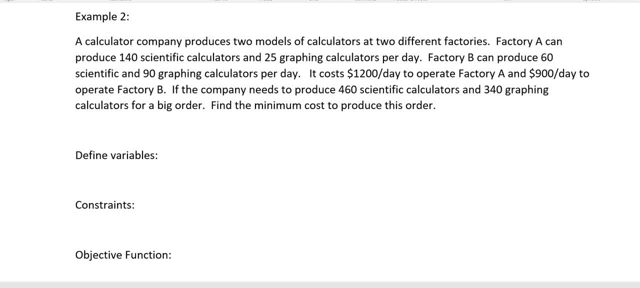 operate factory A and $900 a day to operate factory B. If the company needs to produce 460 scientific calculators and 340 graphing calculators for a big order- sorry, that's not really good grammar or not a good sentence- then we need to find the minimum cost to produce this order. 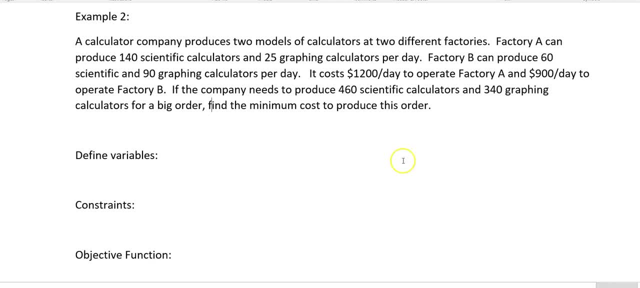 Let's go ahead and just make that Boom, Okay, So right there at the end, I have figured out what it is. I'm supposed to be minimizing or maximizing. I'm supposed to be finding the minimum cost. So that tells me my. 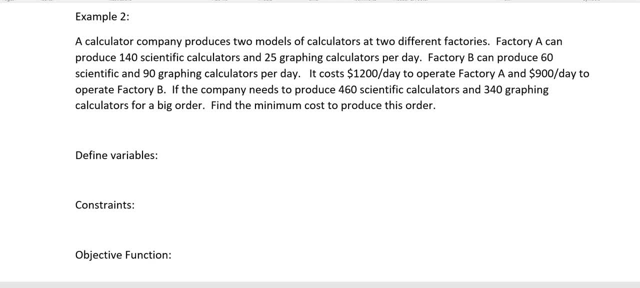 Factory B can produce 60 scientific and 90 graphing calculators per day. It costs $1,200 a day to operate factory A and $900 a day to operate factory B If the company needs to produce 460 scientific calculators and 340 graphing. 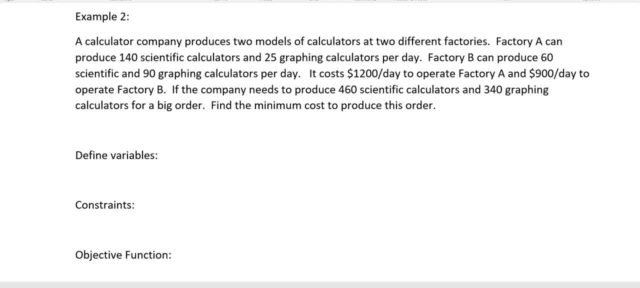 calculators for a big order- sorry, that's not really good grammar or not a good sentence. then we need to find the minimum cost to produce this order. Let's go ahead and just make that Boom. Okay, so right there at the end. 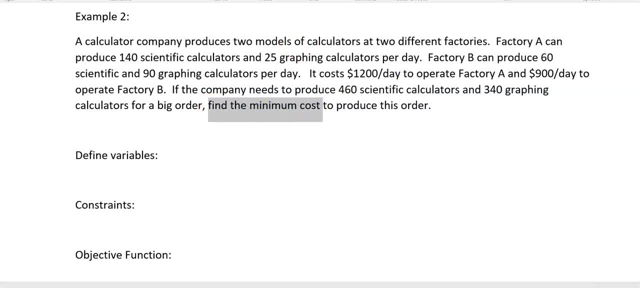 I have figured out what it is I'm supposed to be minimizing or maximizing. I'm supposed to be finding the minimum cost. So that tells me my objective function is going to be about the minimum cost. So it's going to be like how to calculate the minimum cost. 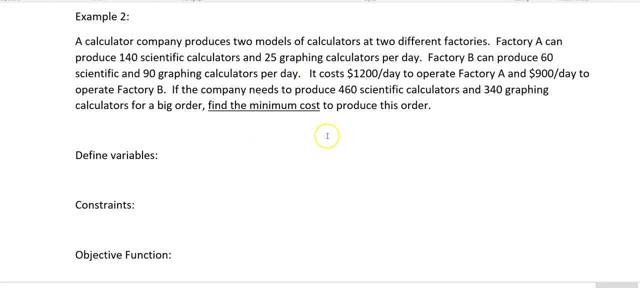 Okay. well, cost is money. So I'm going to go back up here and I'm going to look at all the information about money. Let's highlight that: a different color. It's right there, Okay, so all the information about money is right there. 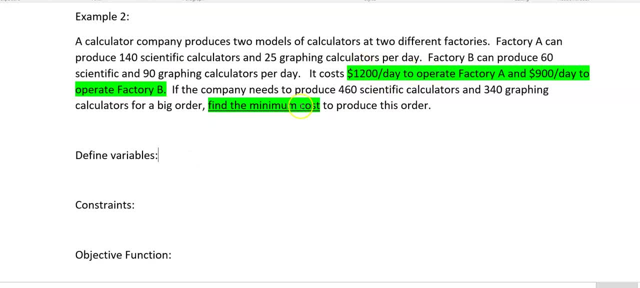 and I need to say I need to figure out how to calculate basically the cost. We don't need to have to figure out how to calculate the minimum cost. We'll figure out at the end of the problem whether it's the minimum or the. 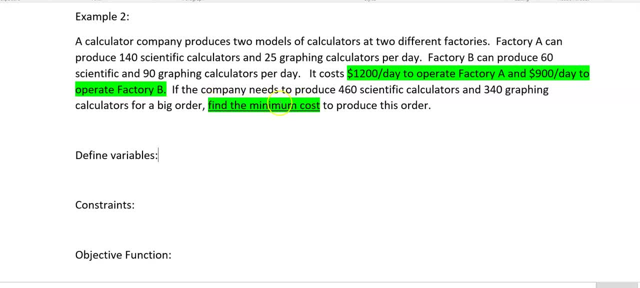 maximum, But just an expression for calculating the cost of producing the business order is what I'm looking for here. Well, since the costs of operating are given in how you know how much it costs each day to operate at factory A and how much it costs. 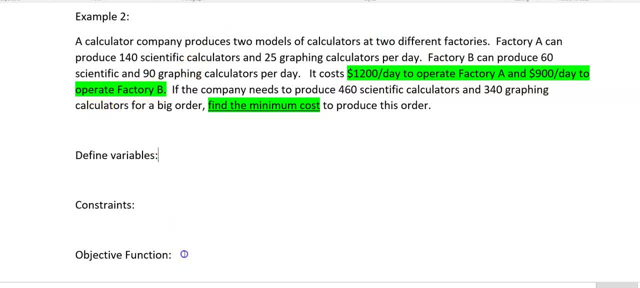 each day to operate factory B, then my objective function is going to be $1,200 per day at factory A plus $900 per day at factory B. That's how I would know how much it cost If I knew how many days factory A was operating. 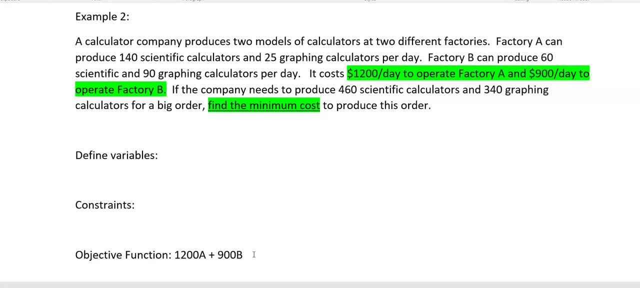 and if I knew how many days factory B was operated, then I could calculate the cost. good night. so once I figure out that's what it would take to know to calculate the fat cost. that's going to be my expression and that also tells me what my variables are going to be about. my variables are going to be about the. 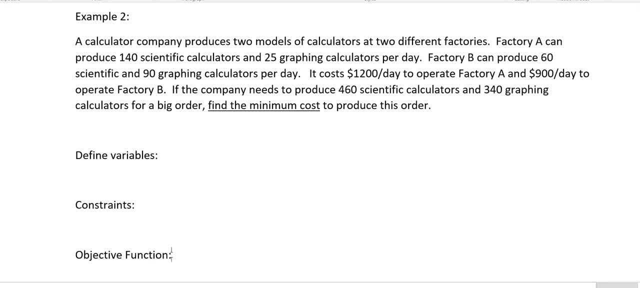 objective function is going to be about the minimum cost. So it's going to be like: how to calculate the minimum cost? Okay, Well, cost is money. So I'm going to go back up here and I'm going to look at all the integrals. So how do I calculate the minimum cost? Okay, So I'm going 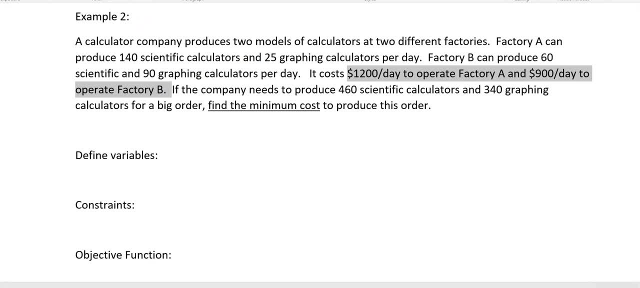 to look at all the integrals. So how do I calculate the minimum cost? Okay, Well, cost is money. So I'm the information about money. let's highlight that. a different color, it's right there, okay, so all the information about money is right there and I need to say I need to figure out how to calculate. 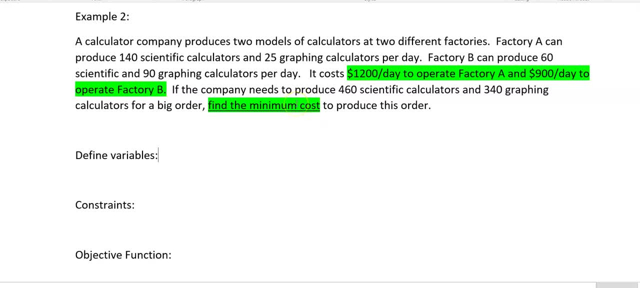 basically the cost. we don't need to have to figure out how to calculate the minimum cost- we'll figure out at the end of the problem whether it's the minimum or the maximum- but just a an expression for calculating the cost of producing this order is what I'm looking for. 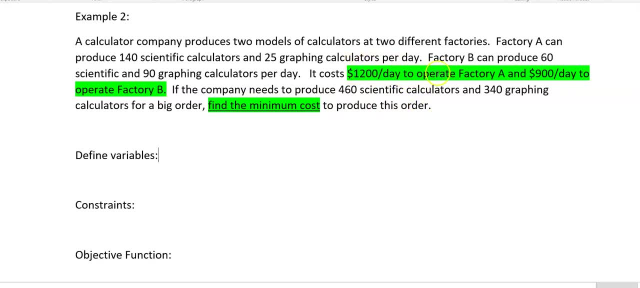 here. well, since the costs of operating are given in how you know how much it costs each day to operate factory a and how much it costs each day to operate factory b, then my objective function is going to be 1200 per day at factory a plus 900 per day at factory b. that's how I would know. 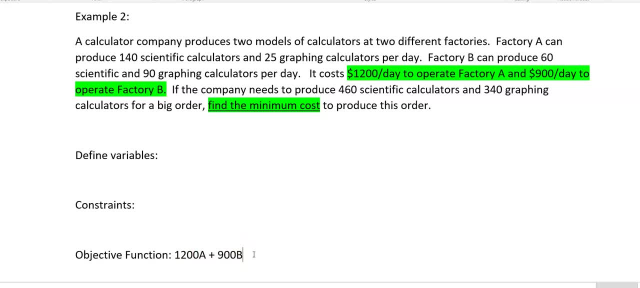 how much it costs. if I knew how many days factory a was operated, and if I knew how many days factory b was operated, then I could calculate the cost, couldn't I? so, once I figure out, that's what it would take to know to calculate the cost. that's going to be my 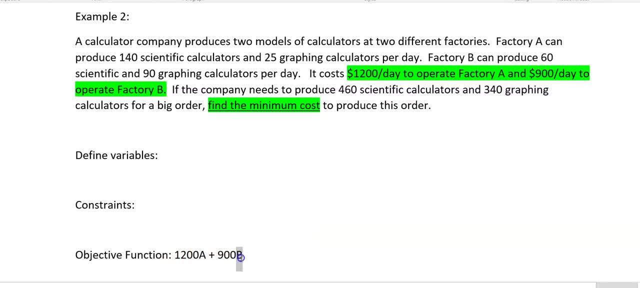 expression, and that also tells me what my variables are going to be about. my variables are going to be about the number of days factory a is operated and the number of days 1, 2. thisonly, in order to get this order done, a number of days of factory a is a and the number of days at factory b is B. 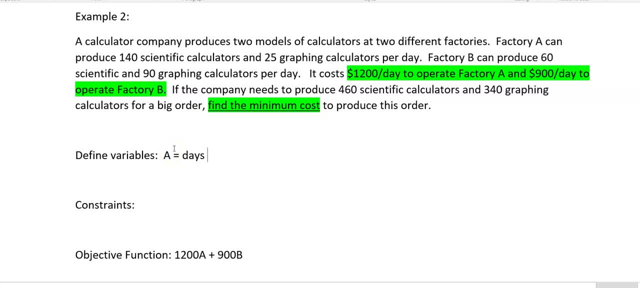 number of days factory a is operated and the number of days factory B is operated, in order to get this order done. okay, so each day at factory a is a number of days at factory area, rather is A, and the number of days at factory B is B. All right, So now one thing: we're very 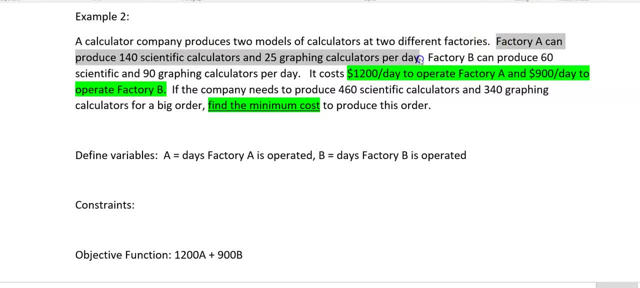 tempted to do with our past math experience is we're tempted to take a sentence and turn it into an equation. All right, But in this case, very often, you're not going to do that. All right. Here's why. A is the number of days for factory A. 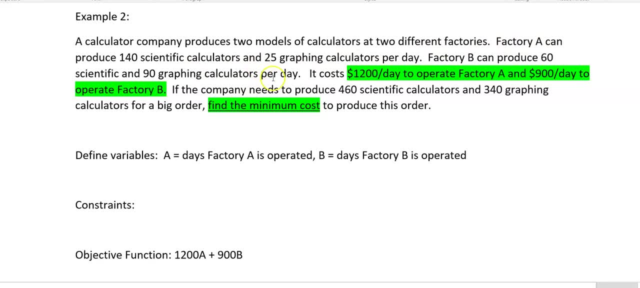 B is the number of days for factory B And basically I have a different type of total here. I know that I need 460 scientific, Okay, So this 460 scientific calculators, that's made up of however many scientific- I mean however many days- factory A is operating. 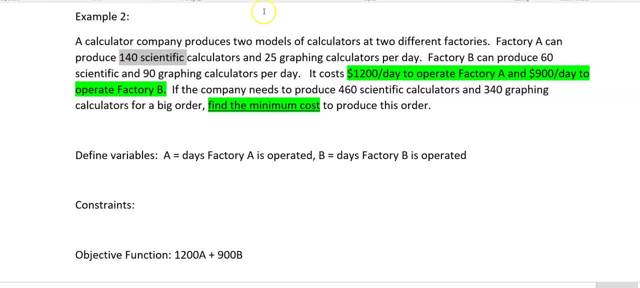 times 140 for each one of those days, plus however many days factory B is operating times 60 for those days. So very often in limiting your programming, your, your um, constraints, which kind of like, kind of like equations. they're inequalities but they're. 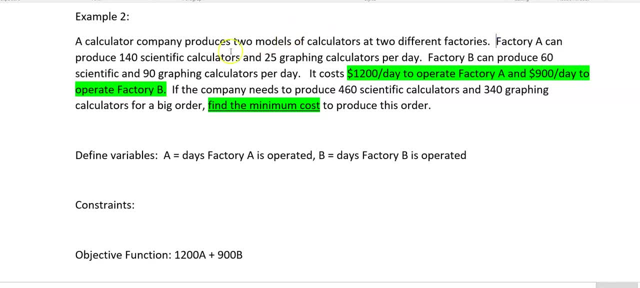 kind of like equations. They don't each come from a single sentence. They come from taking a category and saying: okay, um, 140 scientific calculators per day of factory A plus 60 calculators per day of factory B has to come out to 460. 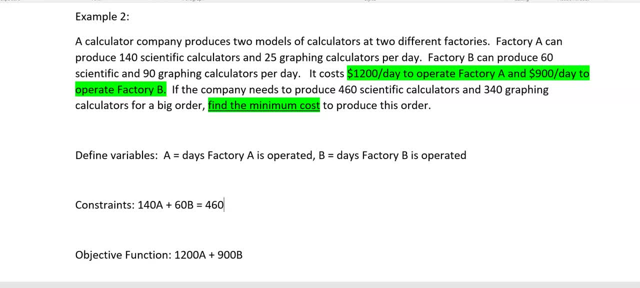 Okay, Then we have what's going on with the graphing calculators. We have 25 graphing calculators per day at factory A plus 90 graphing calculators per day at factory B has to come out to 340.. Okay. 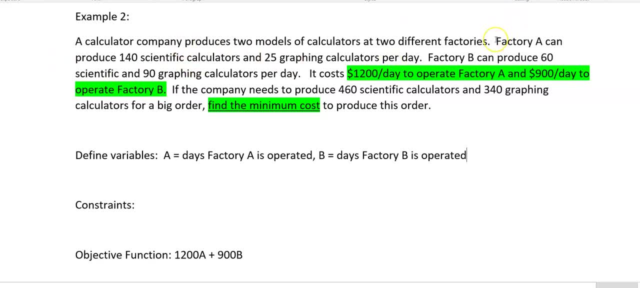 2 celebrate the. we're very tempted to do with our past math experiences: were tempted to take a sentence and turn into equation, all right, but in this case, very often, you're not going to do that. all right. here's why: a is the number of days for factory a, b is the number of days for factory b and basically i. 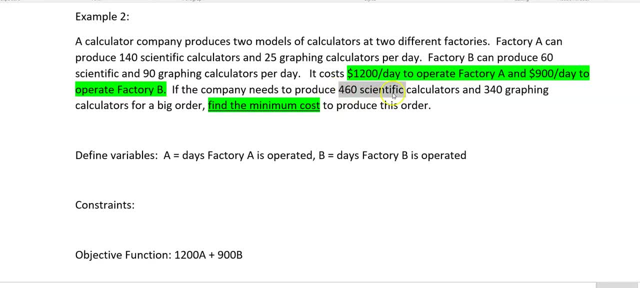 have a different type of total here. i know that i need 460 scientific. okay, so this 460 scientific calculators that's made up of however many scientific i mean however many days factory a is operating times: 140 for each one of those days, plus however many days factory b is operating. 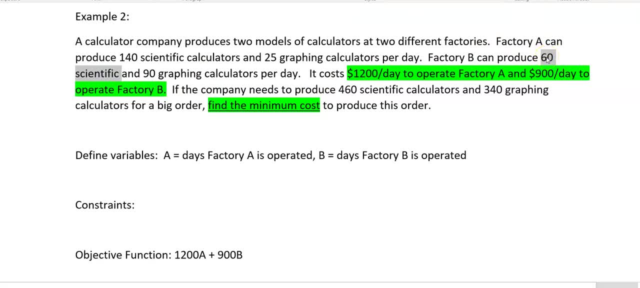 times 60 for those days. so very often in limited year programming, your, your constraints, which kind of like. kind of like equations. they're inequalities but they're kind of like equations. they don't each come from a single sentence. they come from taking a category and saying okay. 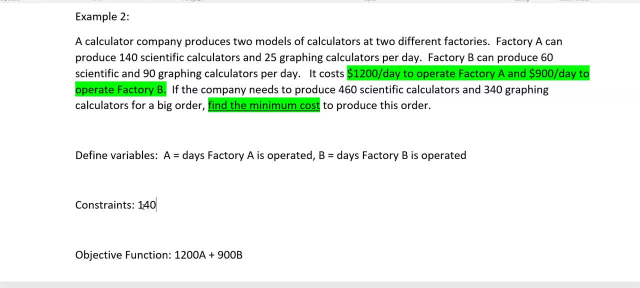 um 140 scientific calculators per day of factory a plus 60 calculators per day of factory b, has to come out to 460.. okay, then we have what's going on with the graphing calculators. we have 25 graphing calculators per day at factory a plus 90 graphing calculators per day at factory b. 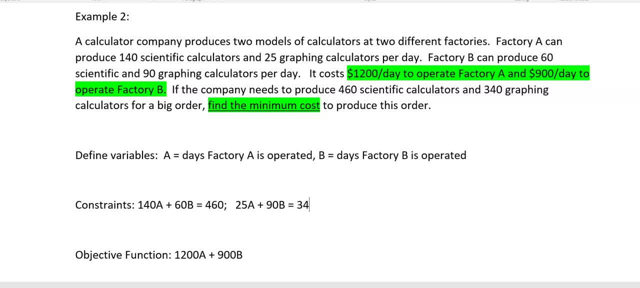 has to come out to 340.. but look at this: notice that i told you that we were always going to have inequalities for constraints. okay, well, those are. those are equations, right, but the deal about that is is, if they produce more because they're not just sending out this order, this is just when. 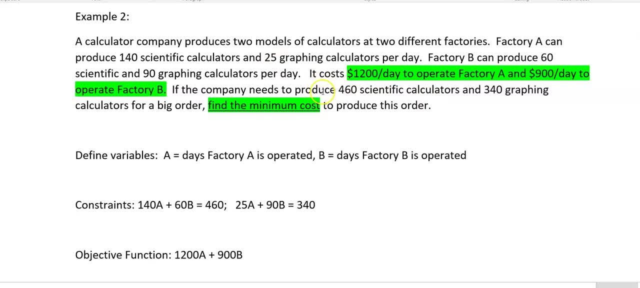 when they'll have enough calculators to produce this order. they'll probably produce more than that on a given day. in other words, it may be that they produce. you know in however many days they've produced 500 calculators. that's enough to send this order out. 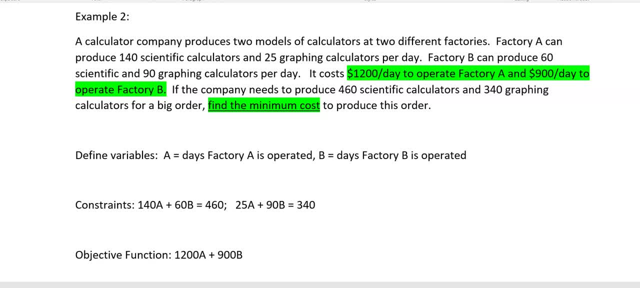 But look at this, Notice that I told you that we were always going to have inequalities for constraints. Okay, Well, those are. those are equations, right, But the deal about that is is, if they produce more because they're not just sending out this order, this is just when. 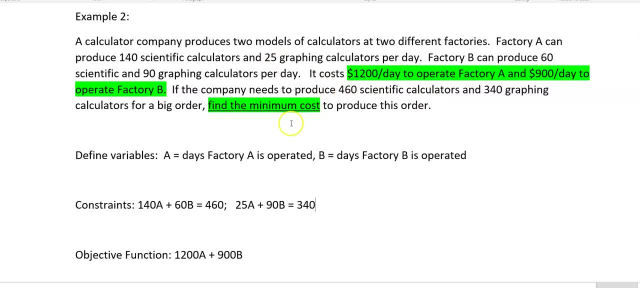 when they'll have enough calculators to produce this order. they'll probably produce more than that on a given day. In other words, it may be that they produce. you know in however many days they've produced 500 calculators. That's enough to send this order out. So really we need. 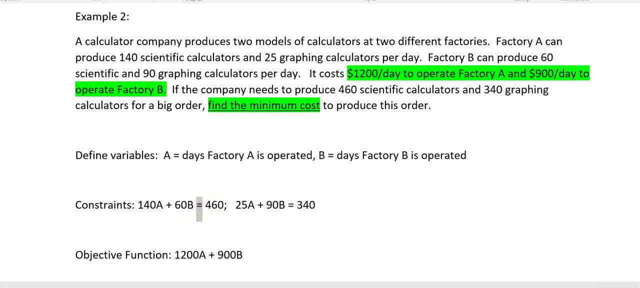 the number of scientific calculators to be greater than, or equal to 460.. And we need this number of graphing calculators to be greater than or equal to 340 in order to be able to send out this order. All right Now, if you don't have many constraints like here, we only have two. 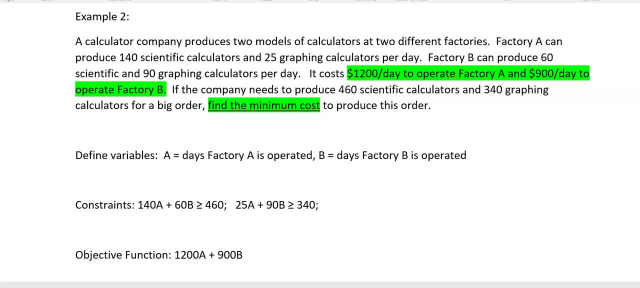 Consider also the fact that we're not ever going to have a number, a negative number of- excuse me- a negative number of days at factory A or a negative number of days at factory B. So we know that the number of days we're producing calculators at factory A is greater than or equal. 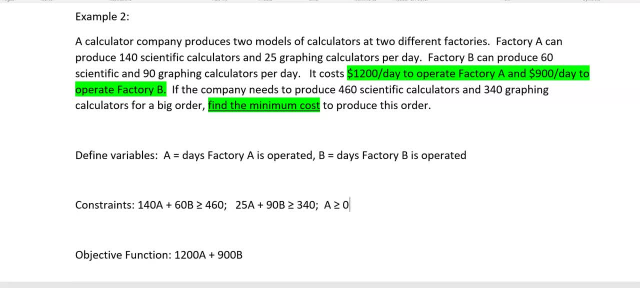 to zero. So that becomes another constraint, And we know that the number of days that we are whoa a little crazy there, Number of days that we are producing calculators at factory B, is greater than or equal to zero as well. So these are my constraints. We'll get into this more later, but you would basically know. 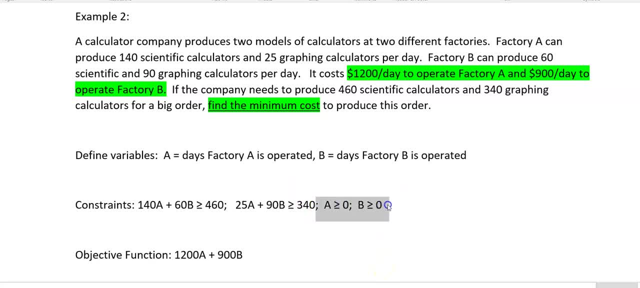 that you needed to throw these in if you graphed your constraints and you didn't have a polygon, basically. So we're going to talk more about that tomorrow. But what you're going to do with all this is you're going to graph your constraints. It's going to give you a shaded area that is like a 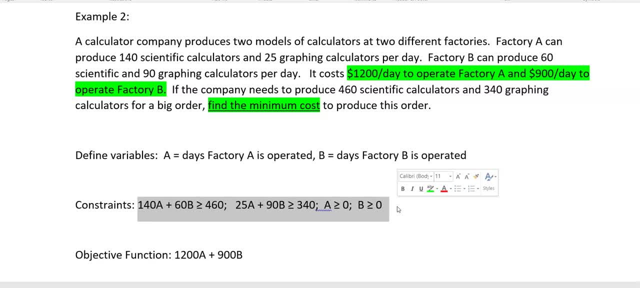 polygon, some sort of quadrilateral, maybe a triangle, maybe usually not much more complicated than that, But it'll give you a polygonal region is what that's usually called, but some sort of shape. And then what you will do is you will look at the corners of the shape and you'll find the 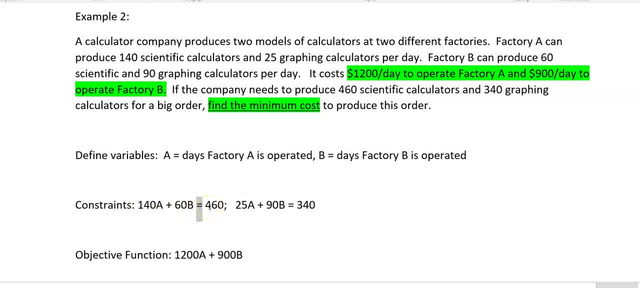 so, really, we need the number of scientific calculators to be greater than, or equal to, 460.. and we need this number of graphing calculators to be greater than, or equal to 340 in order to be able to send out this order. all right now, if you don't have many constraints like here, we only have two. 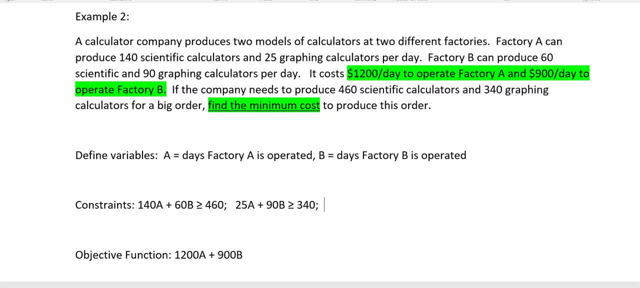 consider also the fact that we're not ever going to have a number, a negative number of science, of- excuse me, a negative number of days at factory a or a negative number of days at factory b. so we know that the number of days we're producing calculators at factory a is greater than or equal. 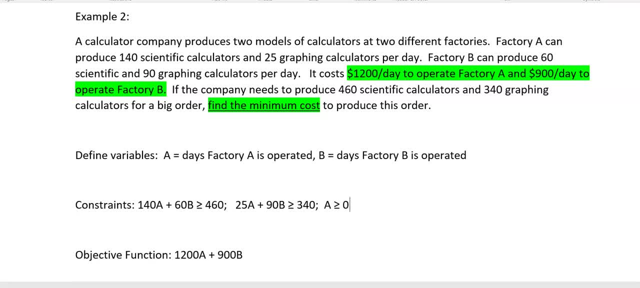 to zero. so that becomes another constraint. and we know that the number of days that we are whoa a little crazy there, number of days that we are producing calculators at factory b, is greater than or equal to zero as well. so these are my constraints. um, we'll get into this more. 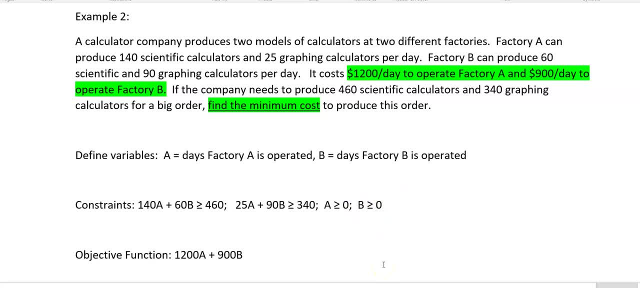 later, but you would basically know that you needed to throw these in if you graphed your constraints and you didn't have a polygon, basically. so we're going to talk more about that tomorrow, but what you're going to do with all this stuff is you're going to graph your constraints. it's going to give. 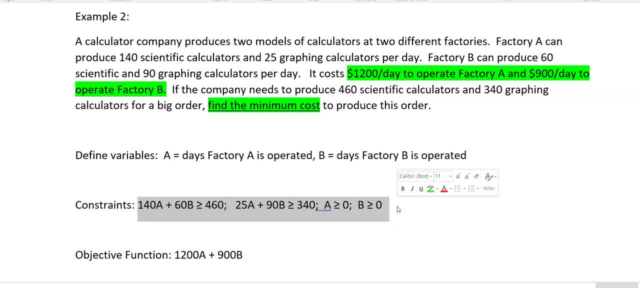 you a shaded area that is like a polygon, some sort of quadrilateral, maybe a triangle, maybe usually not much more complicated than that, but it'll give you a polygonal region- is what that's usually called- but some sort of shape, and then what you will do is you will look at the corners of the shape and you'll find the. 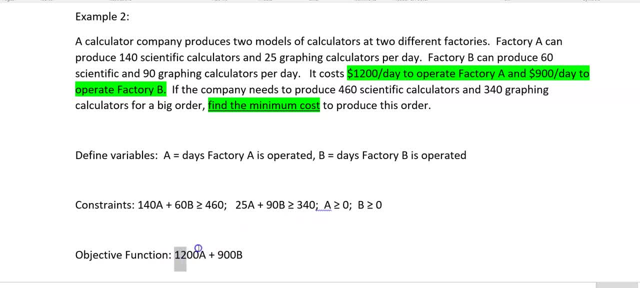 corners of that shape and you'll find the a and the b at each corner and plug them into this. so that's the long range goal. but what you're just doing today is just defining your variables, objective function constraints. so remember, start with your objective function, figure out how you would calculate it and that will help you define. 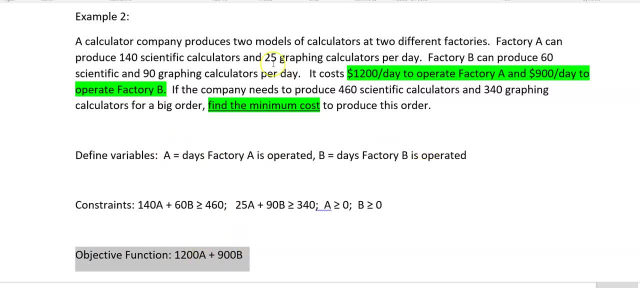 your variables, go, define your variables and then everything else in the problem is going to be some sort of limitation or guideline for those variables and those form your constraints. hope this helps.